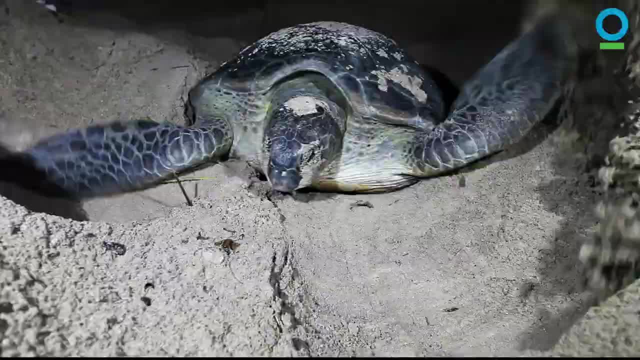 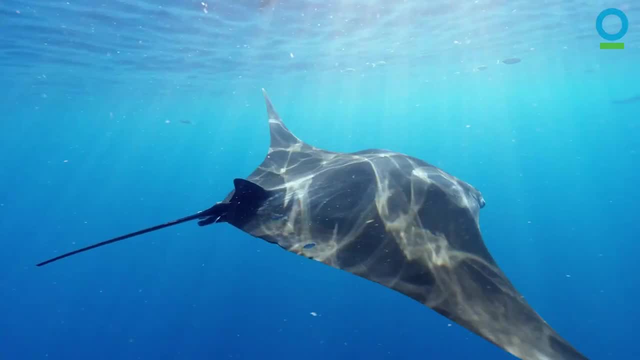 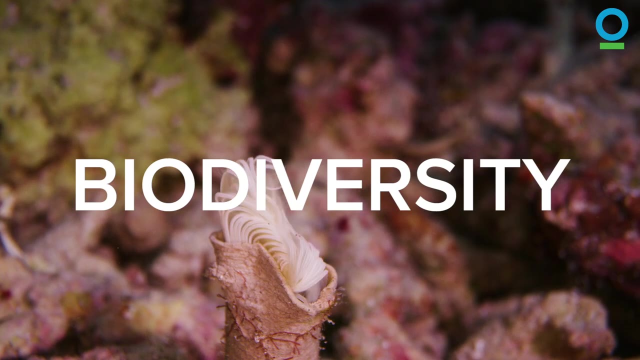 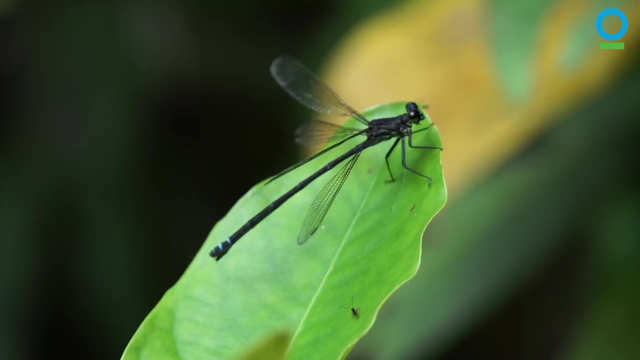 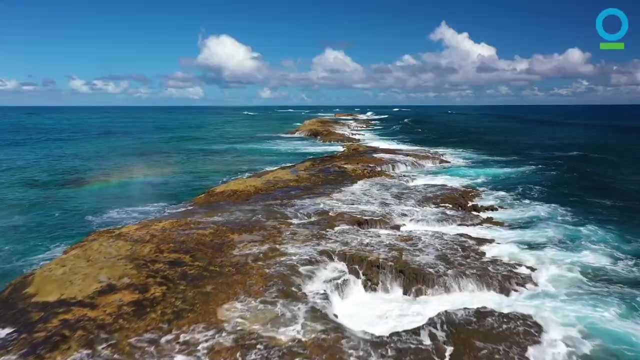 One million plant and animal species are at risk of extinction. The problem is: without this biodiversity, humans are in trouble. Biodiversity is the term used to describe the variety of all life on Earth. Earth's species, their characteristics, even their habitats, are what maintain the health and resilience of nature. 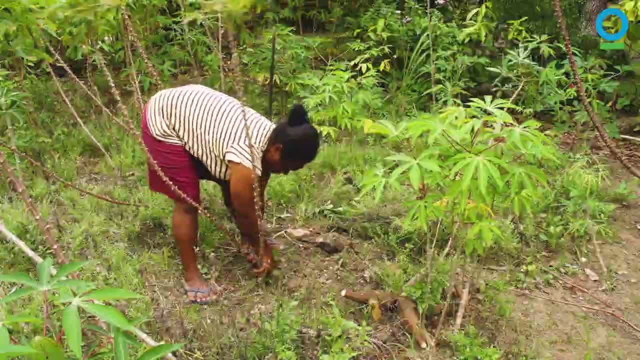 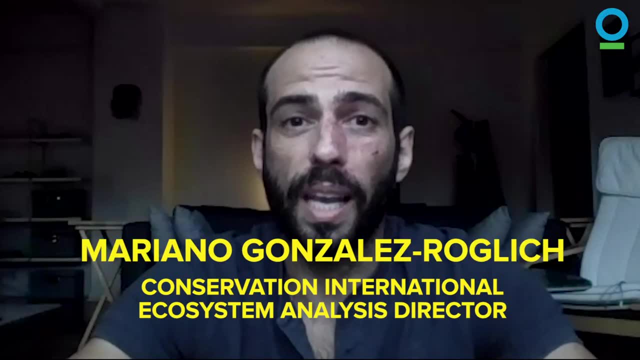 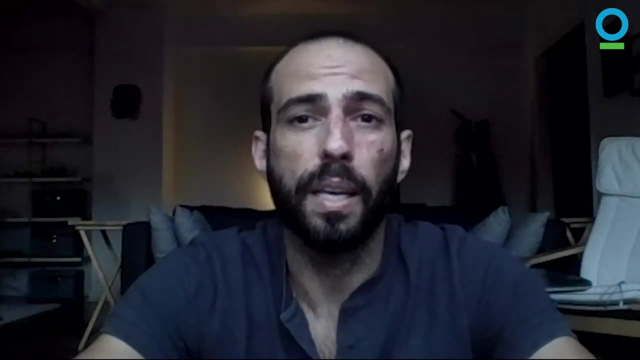 The more biodiversity, the more secure all life is, including ours. Biodiversity is the foundation of all the life on Earth, so we need biodiversity in the form of pollinators to keep our crops growing and to produce the food that we need. We need biodiversity to produce all the medicines that we are needs. We need biodiversity to produce all the medicines that we are needs. We need biodiversity to produce all the medicines that we are, and we need biodiversity to keep healthy ecosystems to suppress the carbon that we need. 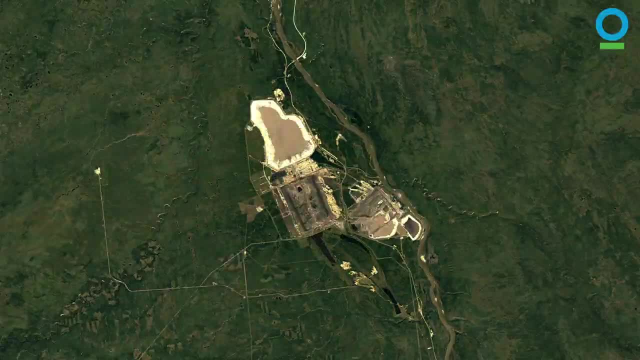 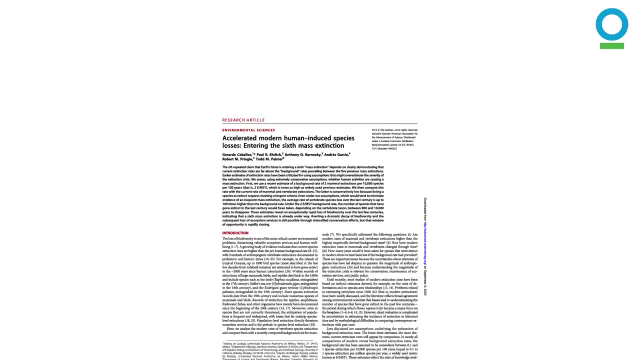 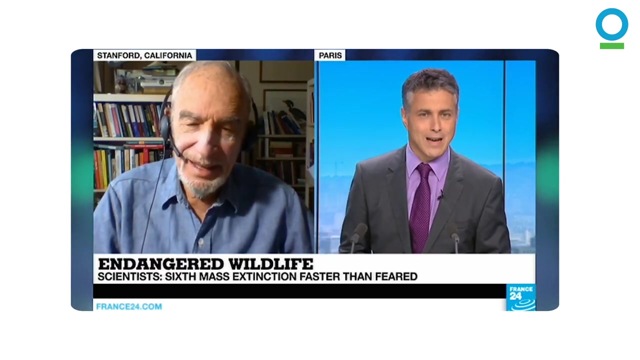 to combat climate change. In the last 50 years, humans have wiped out 68% of animal populations. Experts say that the planet is undergoing its sixth mass extinction, Biggest die-off of life on Earth since the giant meteor that wiped out the dinosaurs. 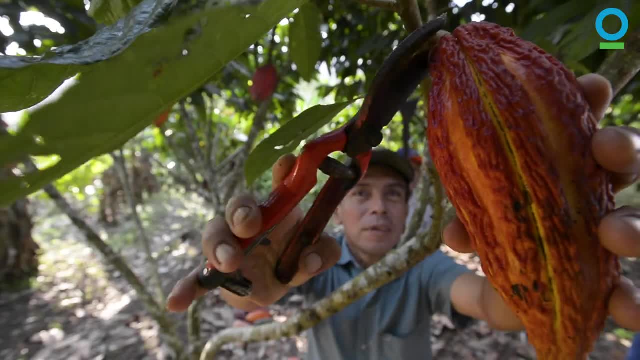 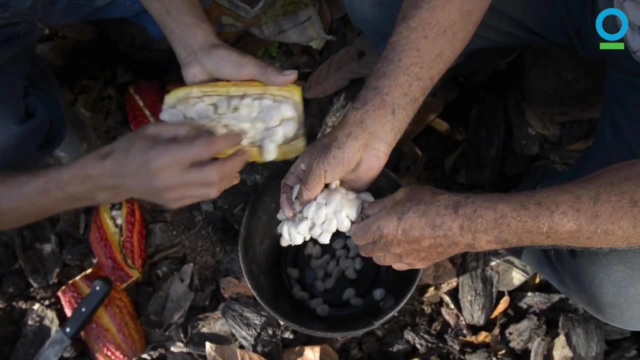 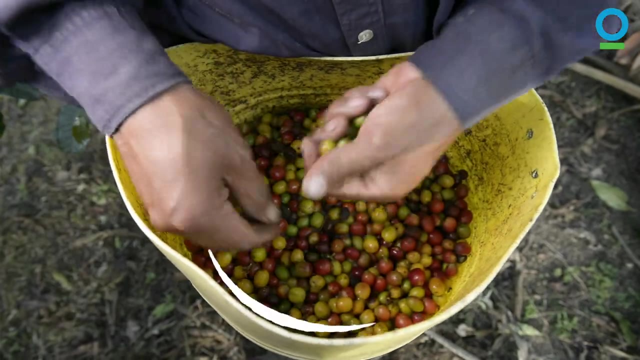 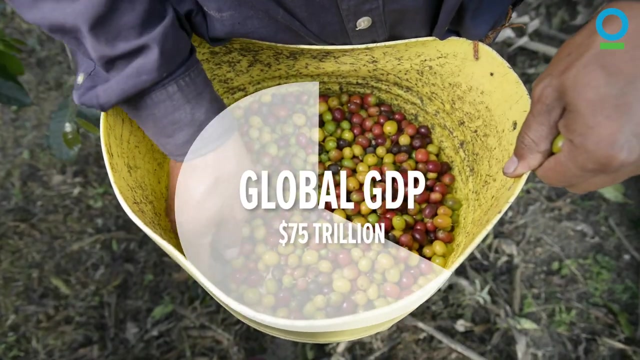 If that doesn't scare you consider this. Biodiversity provides everything humanity needs for free. If we were to put a number on it, the value of goods and services provided by biodiversity is estimated to amount to $125 trillion per year. That's more than two thirds of global GDP. 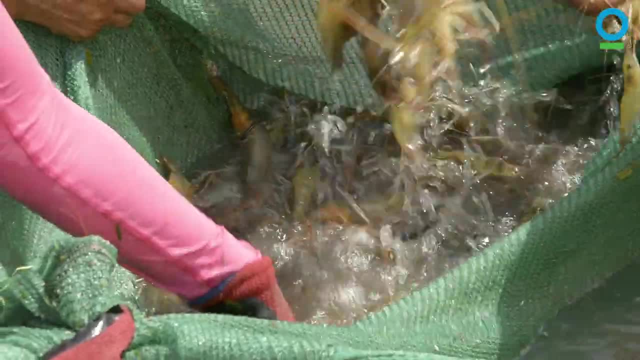 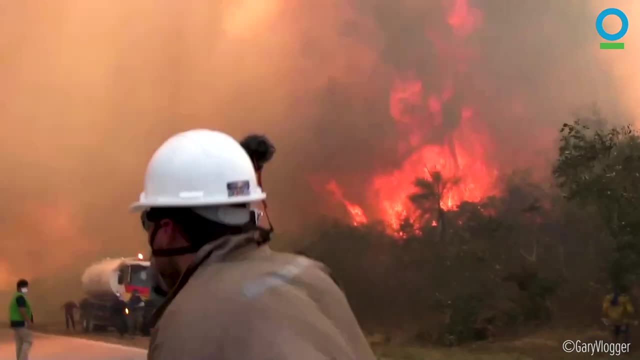 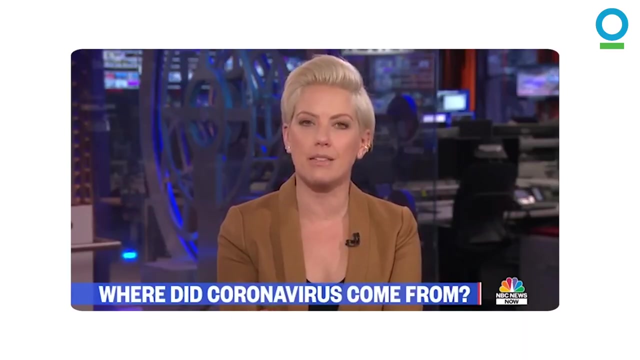 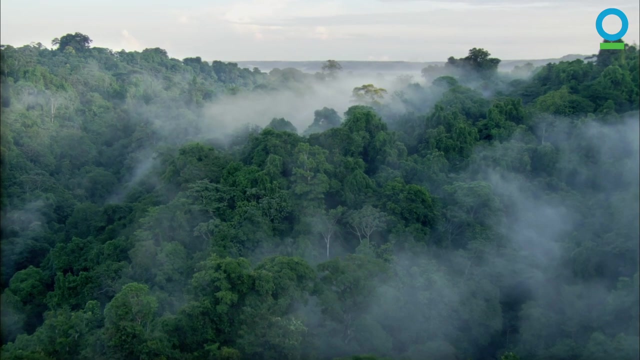 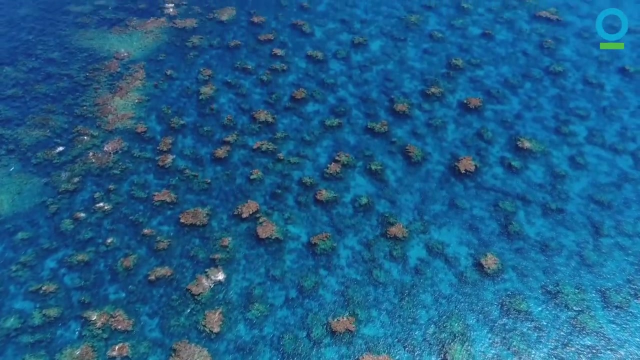 The continued loss of biodiversity affects the food we eat, the water we drink, to say nothing. The Conservationists say that protecting at least 30% of land and 30% of sea on Earth by 2030 is critical for stopping and reversing biodiversity. 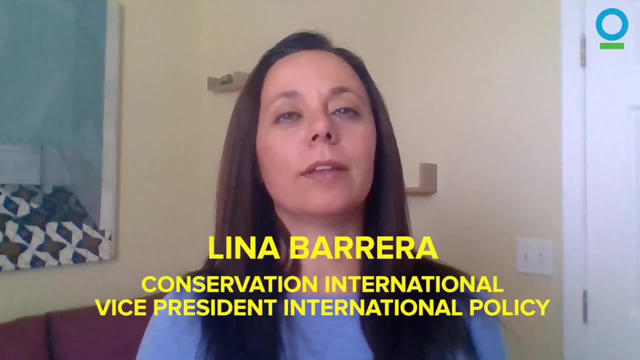 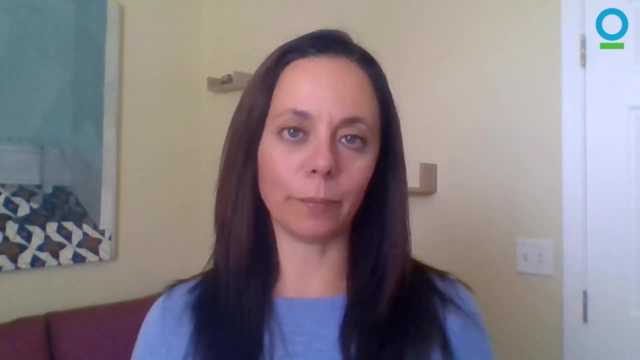 and reducing the loss of species around the globe. The good news is that there's a whole suite of tools that we can implement. It's not just about creating national parks and protected areas, although that is important. It's also about integrating the economic value.